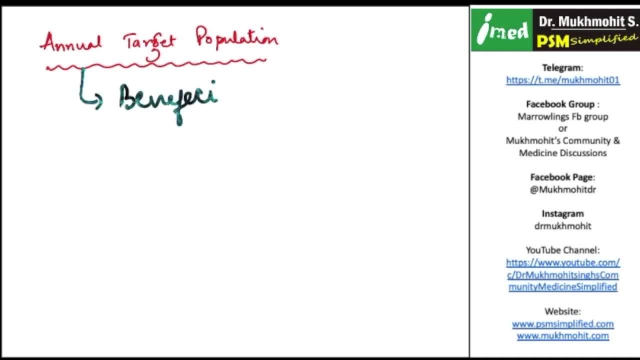 target population, That is, the eligible number of beneficiaries under the program for that particular year. So the beneficiaries could either be the pregnant females where you want to give them the tetanus and diphtheria toxoid vaccine, TD vaccine, or they could be the infants, to whom 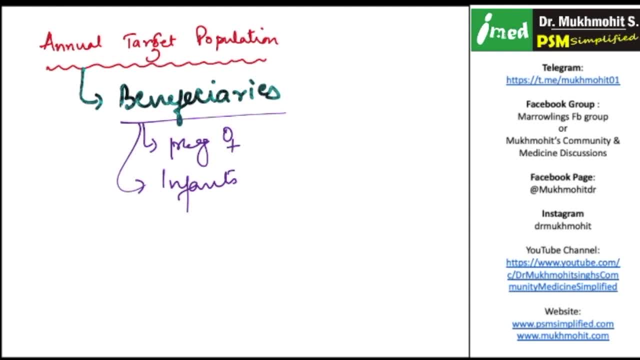 you are going to give the pentavalence or the measles rubella vaccine, or any vaccine for that matter, or it could also be the number of live births where you are concerned for giving them the BCG vaccine. So to know more on how to find out the eligible beneficiaries, you can please visit this YouTube. 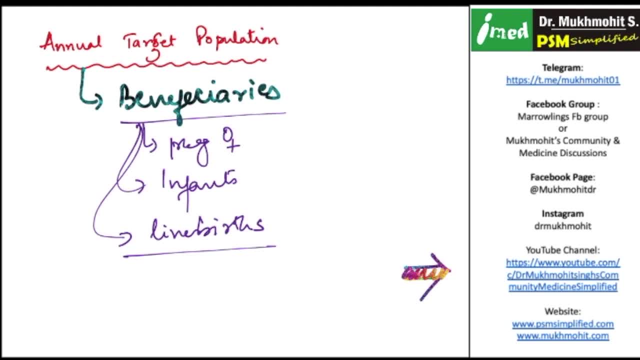 channel that is Mukmohit's Community Medicine Simplified, and in this YouTube channel there is different playlists, So you can find a playlist by name of MCQ Discussions and within that playlist, within this playlist, you need to search for the demography module. Demography module, where you can. 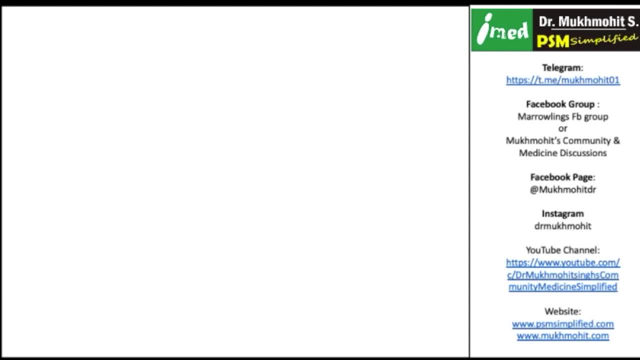 find out how to find out the eligible beneficiaries. So you can find out how to find out the eligible beneficiaries Now, taking a live example that let us say in the rural training health center where I work roughly. just to take it on easy basis, let us say that the total infants which are there in 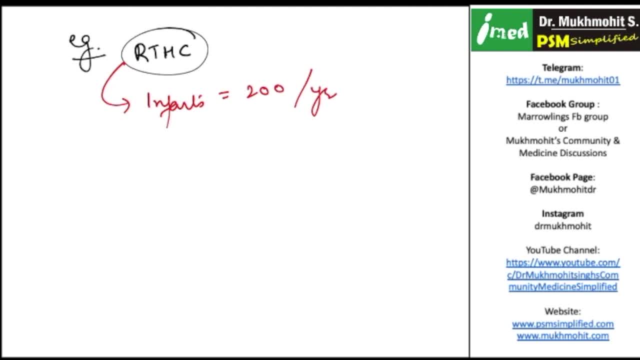 my area is 200 every year. So that is also the data. You can also take the data directly available from the Ministry of Health and Family Welfare or you can do your own calculations and which I have already shown you on the YouTube channel. So, anyways, let us say that the total infants in my area are approximately 200 every year. I want to 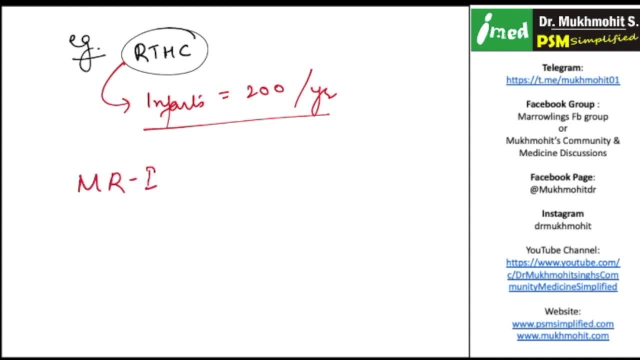 find out what is the vaccine coverage for my measles rubella 1 vaccine or the measles conjugate vaccine 1, which is given at 9 months of age. So what I do is I find out how many total number of infants who received the dose. Let us say in my area there were 160 doses of measles vaccine was. 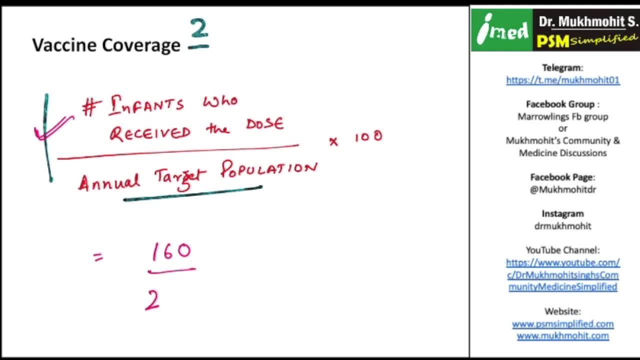 used in last year. So let us say that the total target population, that is 200 multiplied by 100.. So that gives me a vaccine coverage of approximately 80%. This will give me a vaccine coverage of my measles rubella 1 for the. 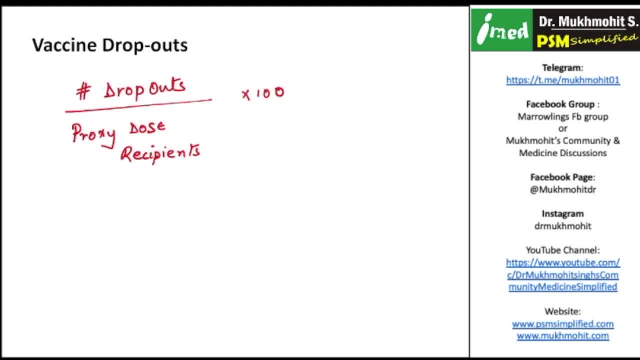 measles: first, vaccine of 80%. Next, let us say how to calculate the point number three, how to find out the dropouts. Now, dropouts are interesting. that simple formula is that you find out the total number of dropouts divided by the proxy dose. 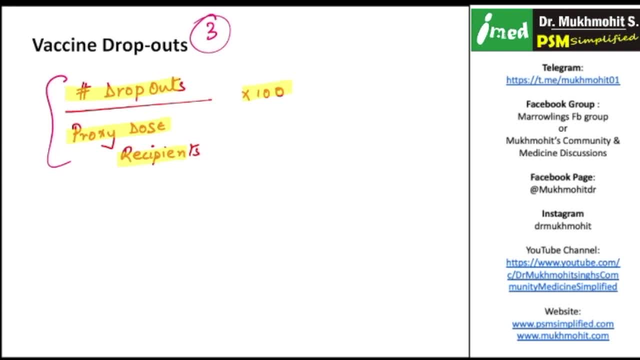 Recipients in 200, simple. But the point is, what do we mean by a dropout? Dropout means that the patient was, or the person was already in the program and he dropped off right. So that means there has to be a proxy dose receipt. For example, I want to find out the dropouts for pentavalent. Usually we take for 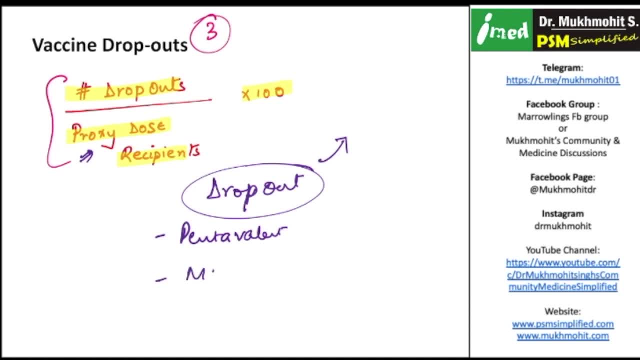 pentavalent. or we find out the dropouts for measles rubella vaccine. So you give measles one and you give measles two, Then you find out the dropouts. So for example, let us say that measles rubella one vaccine was given in my 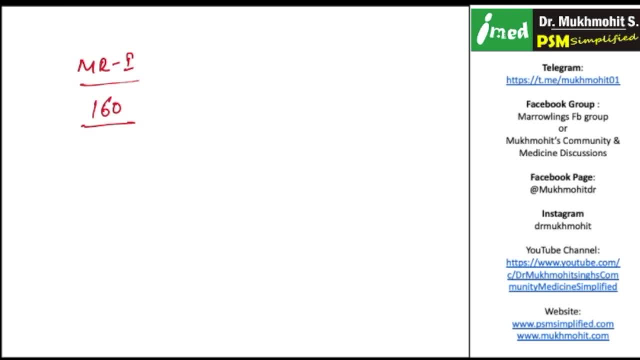 area to 160 children, as we have seen in my previous example also. And the measles rubella two was given to maybe 140 children. So now the dropouts. So now the dropouts are this one minus the two, So one minus. 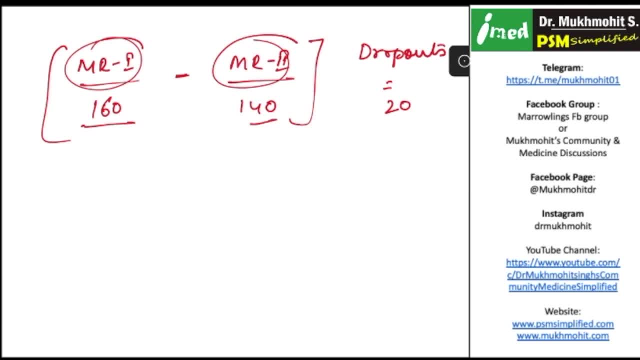 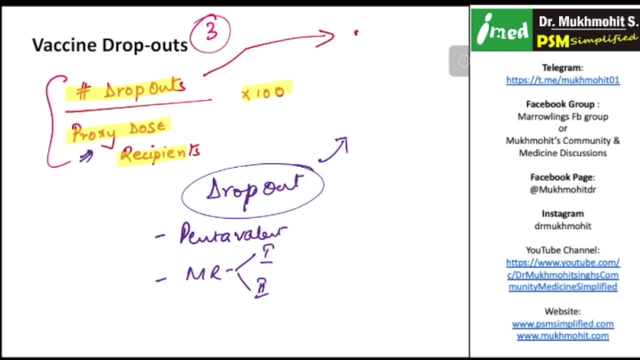 two. So that means the dropouts in my area. So once I get the dropouts, this will be the numerator. This will be the numerator of my formula. So dropouts is equal to 20.. And what is the proxy dose recipients? We know that the proxy dose recipient, that is the first dose recipient, first dose. 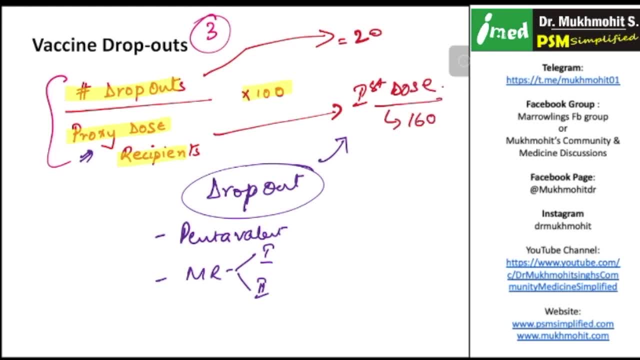 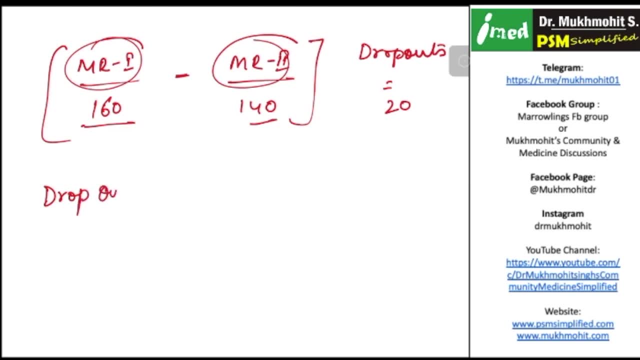 So that was you remember was 160.. So what is the dropouts over here? The dropouts will be calculated as, So the dropout rate will be calculated as 20.. So we have say 60 by divided by 160 into 100. So that will come out to 6 to 12. So 12.5% will be my dropout rate. That's how you calculate the dropouts. There is a slight variation in this whenever we're calculating the dropouts, So usually we have to take a proxy vaccine indicator. So therefore, for oral polio vaccine, you will take the first dose. You have your O Penceburton RBS vaccine. And we have ticked a different number for a drug, in this case SARS Endaming. If it's a different sample, we will start cross radi, shockinggo or other viruses, Just likeECTU. Just likeECTU To use that same Batamble extraction, or even plus Biron vaccine.